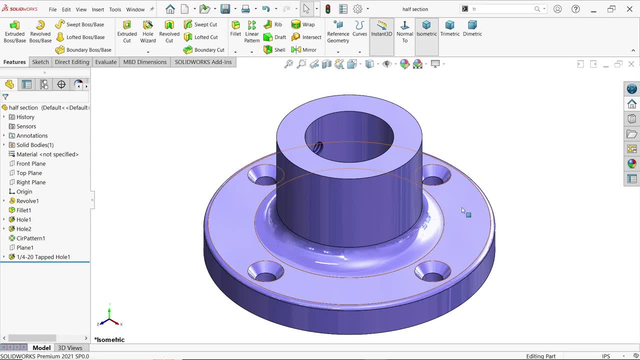 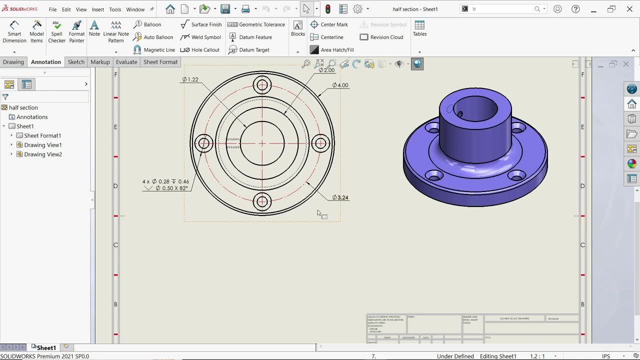 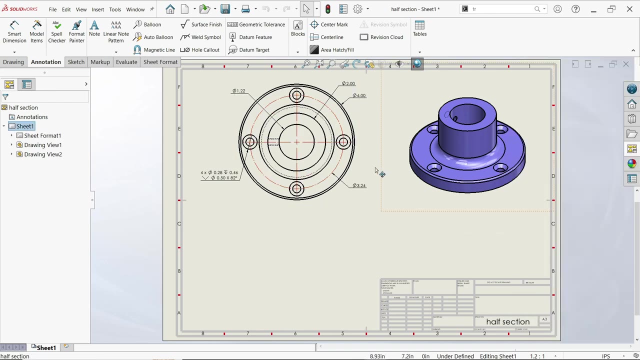 How to make half section view in solidworks drawing. So this is our model. I already made one drawing. This is top view. If you check here, this is our top model. Now how to create half section view. for this Half section view is normally used to show a hidden line or 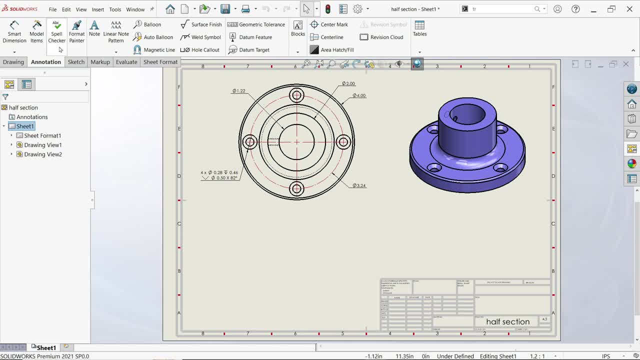 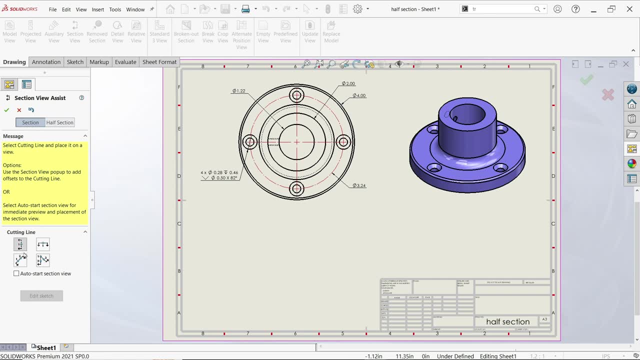 hidden features or hidden dimensions. So if you go to drawing, activate section view and here you will see full section, It is actually a full section, these cutting lines, But just there is an option called half section. Now, here you will see there are many options. 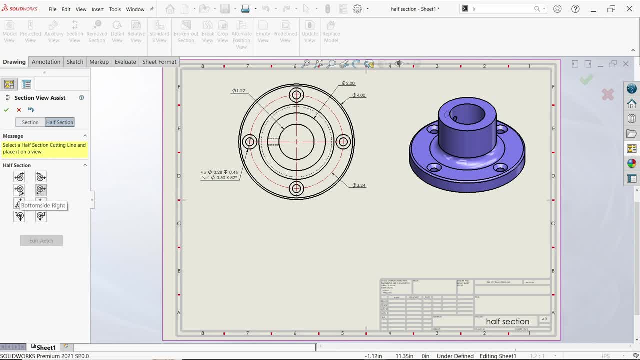 Top side, right left. This is bottom side, right left. Now this is left side down, left side right, Right side down, And this is going to be left side up, left side. So, let's, I am going to choose this one. This is going to be perfectly suits. Now look, you will see the arrow. Select. 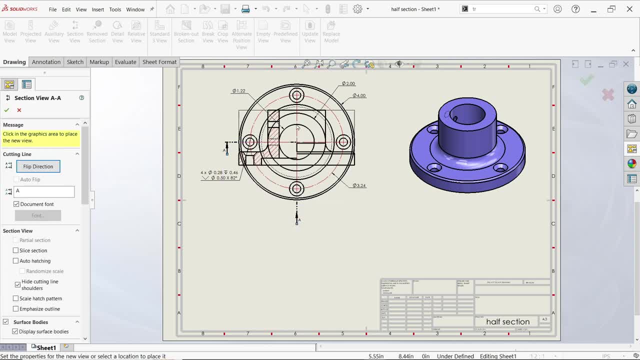 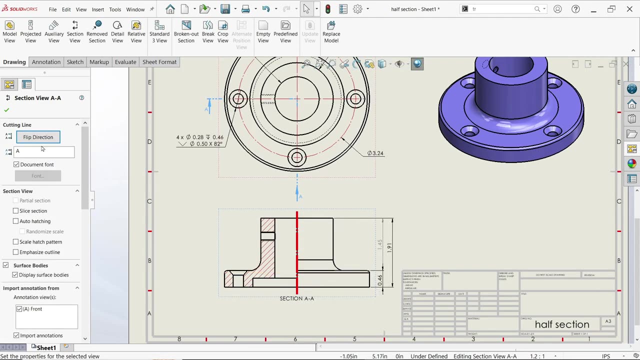 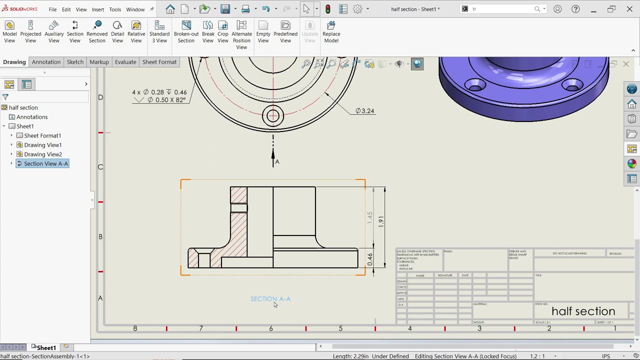 center one and look, the view is created. Now, if you choose flip direction, it will change direction and flip direction. Now look, just simply delete this. Now look, if we check this and here comes slice section view, it will show you only this slice section view. Uncheck auto hatching- already there. 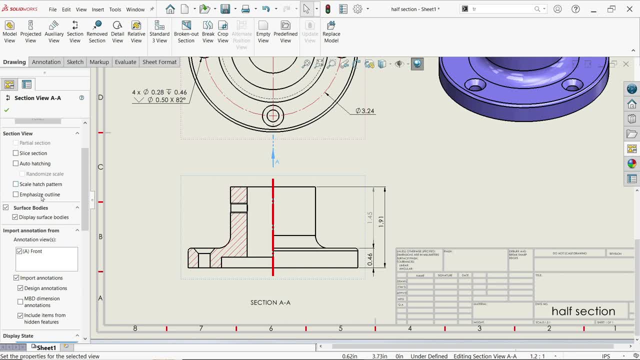 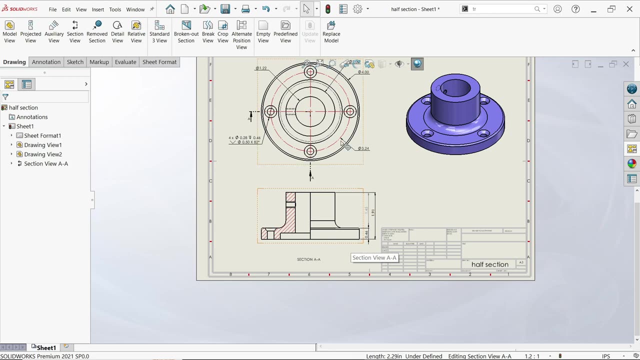 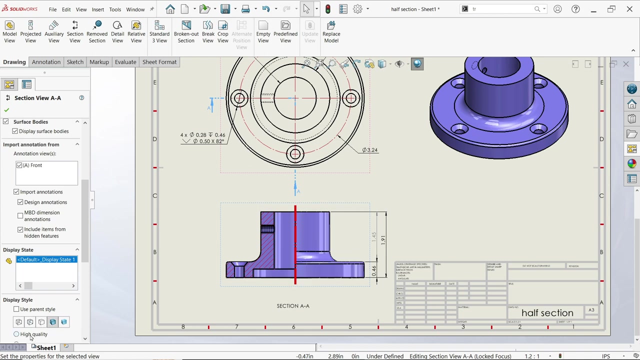 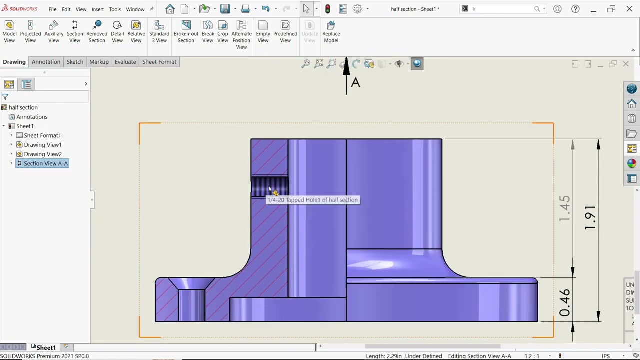 Now scale hatch pattern. but we don't need Emphasize outline. This is already a thickened line, so no need to show And rest, keep as it is. See, even though let's say this view high quality, and you will see here. look, this is a thread. 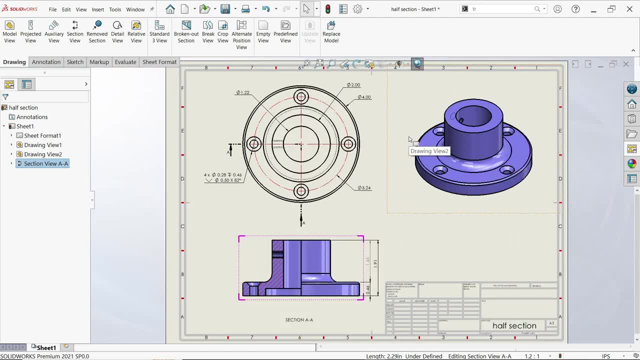 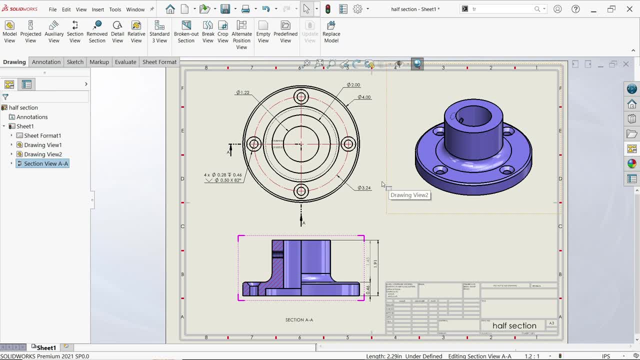 Don't forget to share and like our video and please subscribe our channel for more video and more projects in solidworks. Thanks for watching.